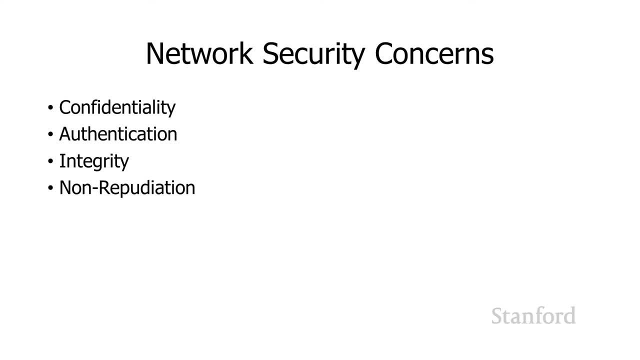 And non-repudiation- being able to determine whether or not somebody actually carried out a particular action in a way such that they can't repudiate it- And the mechanisms we're going to be talking about now are going to take care of these different problems. 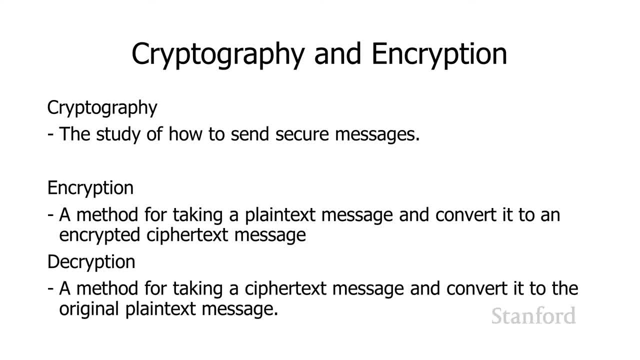 These all fit under the general umbrella of cryptography, which is a study of how to send secure messages. They're going to depend on encryption techniques. encryption means to take a plain text message and convert it to an encrypted ciphertext message, and decryption, which is the reverse process. 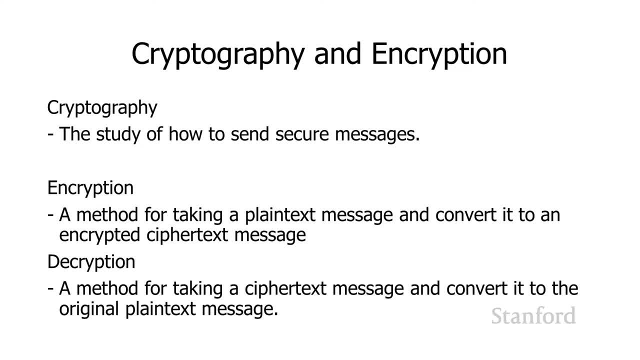 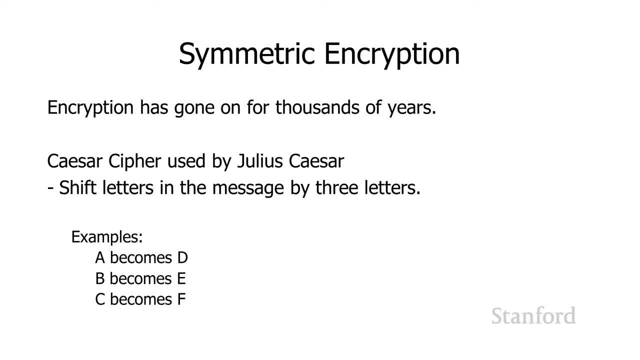 taking the ciphertext message and converting it back to the original plain text. Now we've been doing encryption for thousands of years, And so I'm going to start off by showing you how the Caesar cipher works. This is a pretty simple cipher that you'll all 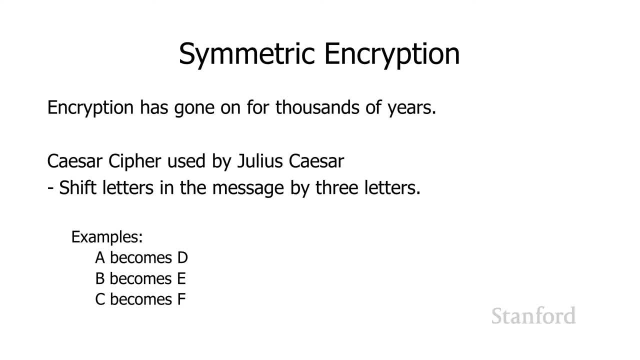 be able to understand quite easily. And it was used by Julius Caesar. So you can see we've been encrypting for quite some time. OK, the way the Caesar cipher works is we shift letters in the message by three letters. So if I've got a message and I've 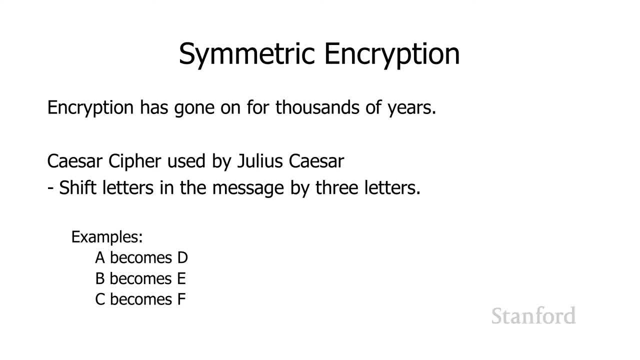 got the letter A in the original text. I'm going to go ahead and shift that A, B, C, D And instead of writing the A, I'm going to write a, D. Instead of writing a, B, I'm going to say B, C, D, E. 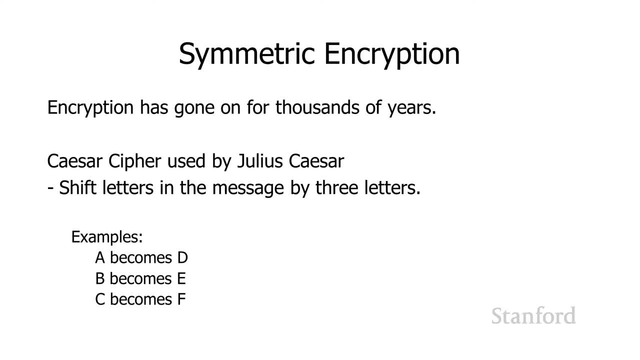 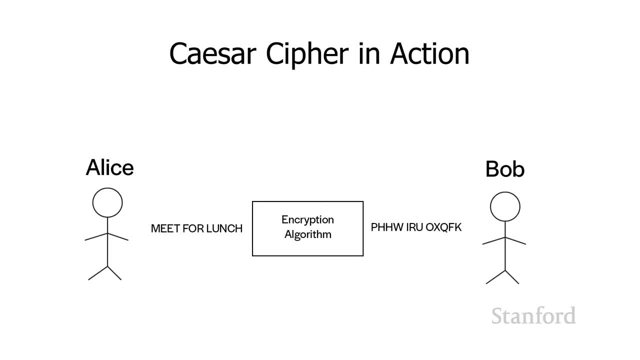 OK, if I shift B over by three characters, I get an E, And so I'm going to write an E instead of a B, Going to write an F instead of a C, and so on. All right, so let's take a look at the Caesar cipher. 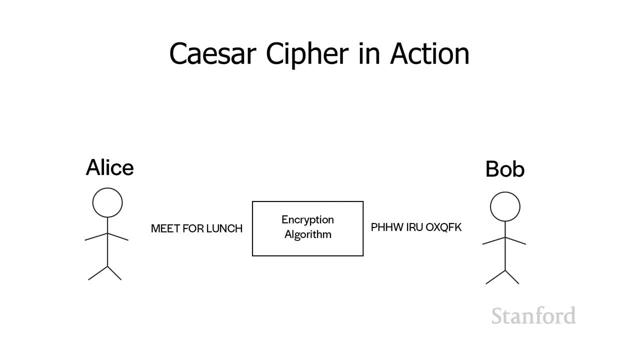 in action. So suppose the TAs are unhappy with how I'm running the class And they decide that they are going to meet for lunch and plot a coup d'etat. So they're concerned because they know I'm a tyrannical guy. 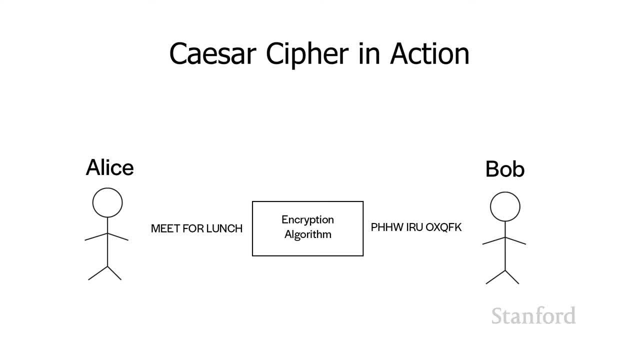 So they don't want me to know that they're meeting And so they're going to take their message here: meet for lunch, And they're going to encrypt it using the Caesar cipher, So the M if we shift it over by three MNOP. 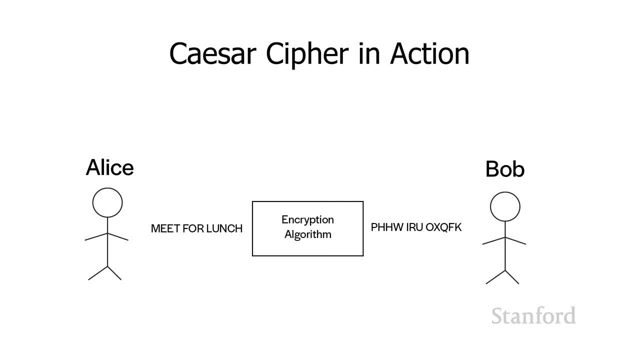 The E becomes EFGH, The T becomes TUVW and so on, And so you can see that meet for lunch becomes PHHWIRU0XQFK. And just again as a reminder, we refer to the original text. 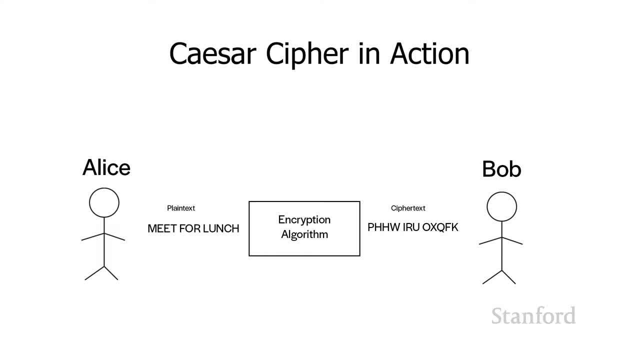 as plain text And the converted text as ciphertext. Now I play the role of Mallory here. I'm the bad guy, And so I intercept the TA's texts And I see PHHWIRU0XQFK. I think. huh, I seem to recall IRU stands for something. 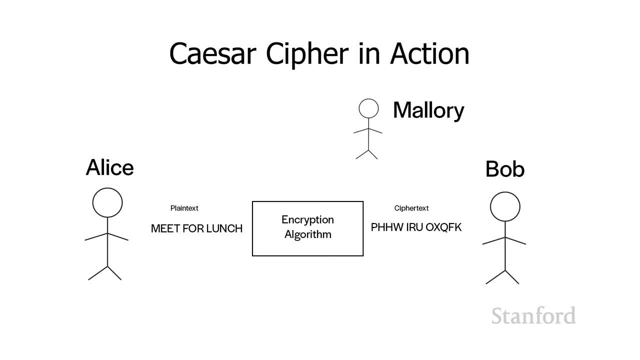 This must be some newfangled kids internet speak. I guess they're just having fun. I have nothing to worry about. Everything's going great, And so the TAs are able to meet for lunch and replace me, And they will be teaching lecture shortly. 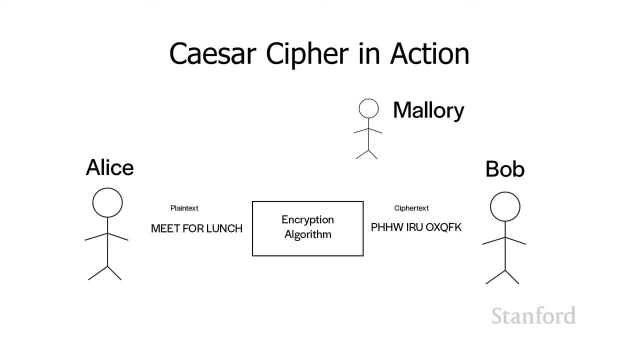 This is actually a true story, Because Ivy, who is one of our TAs, will be teaching the lectures on artificial intelligence, because she is far more of an expert on modern artificial intelligence than I am. I actually have a master's degree in artificial intelligence. 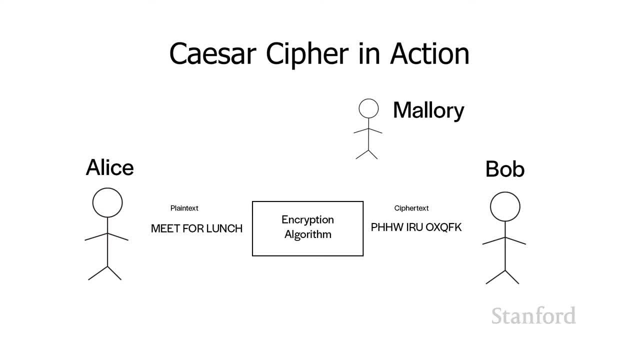 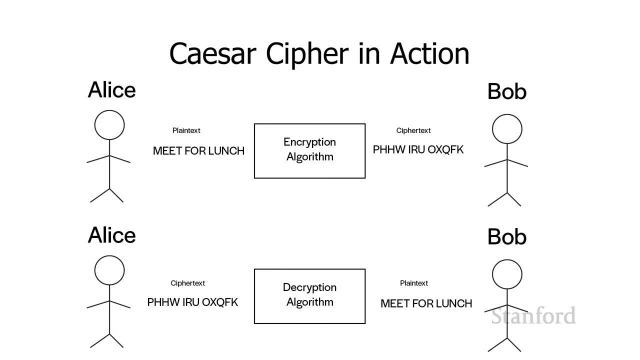 but it's from 1986. So I think things have changed a bit since then. All right, anyway, back to the Caesar cipher. All right, so just as a reminder, we have encryption and decryption. So Alice is going to start with the plain text. meet for lunch. 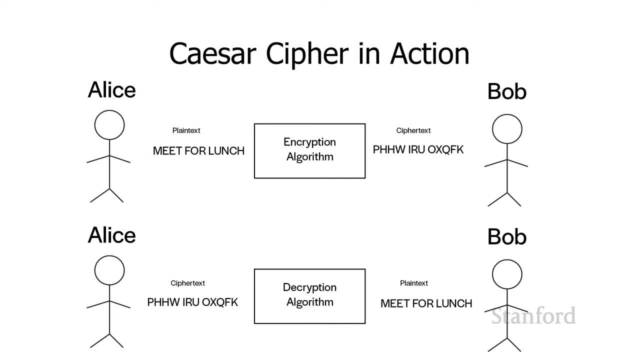 She's going to generate the ciphertext PHHWIRU0XQFK, And then, when Bob receives that ciphertext, he's going to have to pass it back through the decryption algorithm in order to understand what the heck Alice is actually trying to tell him. 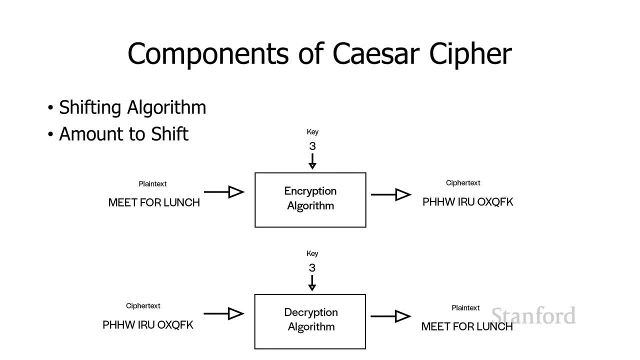 All right, if you think about it, there's actually two components to the Caesar cipher. There's the general shifting algorithm and then there's the amount to shift. So apparently, Augustus Caesar actually used the same shifting algorithm as Julius Caesar did. 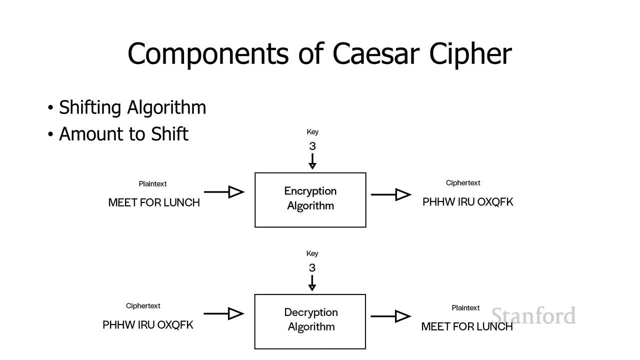 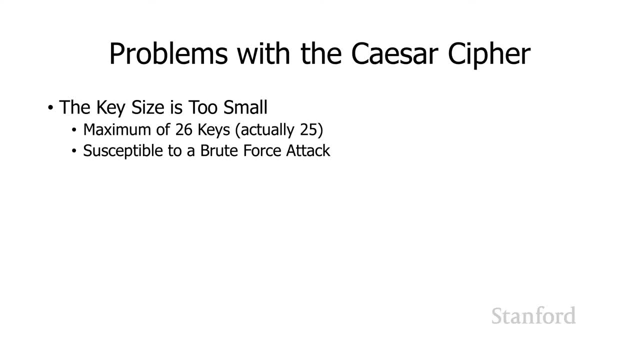 but he changed the amount to shift. It's still shocking to me that their opponents could not figure out the cipher, but they did. Which brings us to the next question. why am I shocked that the cipher actually worked? Because there's a lot of problems with the Caesar cipher. 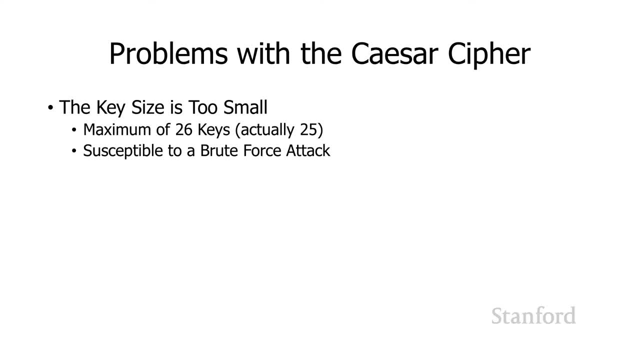 The main one being the key size, is way too small. If we're using English letters, you can only shift up to 26 characters And in fact the 26th character actually rolls around to the original character, So arguably you only have 25 characters. 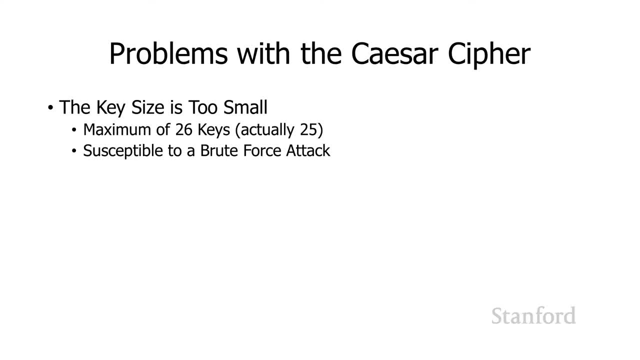 because the 26 is useless, And so this is susceptible to what's called a brute force attack. And so the idea behind a brute force attack is: I just try all the different combinations, Combinations of characters until I use one of them and it results in something that looks like normal English text. 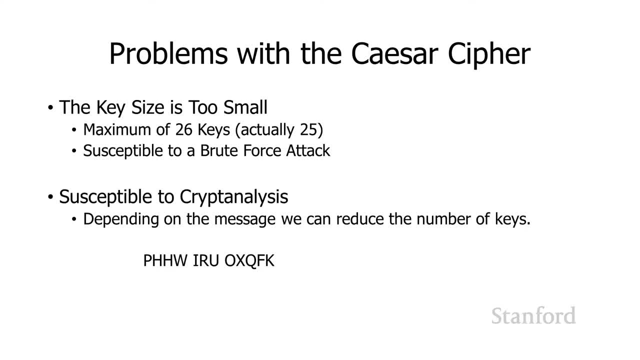 I'm like, oh, that must be the meaning of the message. But it turns out that the Caesar cipher is not just bad because there's only a very limited number of keys, It's also bad because it's susceptible to cryptanalysis. And so what cryptanalysis means is 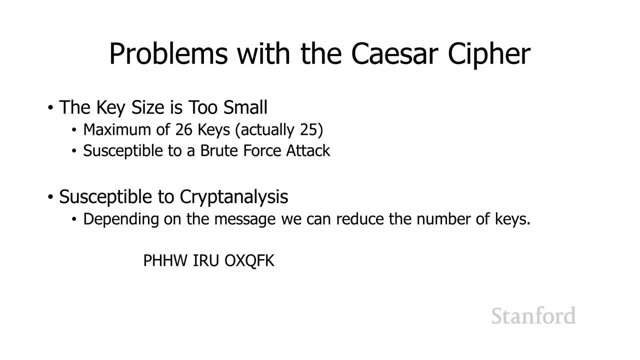 that we take a look at the cipher text and we're able to discern information about the message. We're able to discern the key just by looking at the text, And so, if I look at this text- P-H-H-W-I-R-U-0-X-Q-F-K. 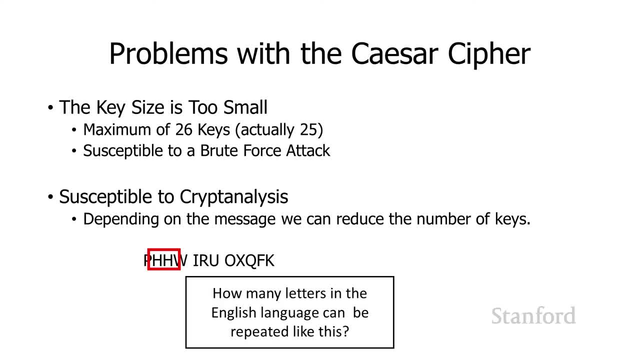 the thing that immediately stands out to me is that pair of H's next to each other. Now, how many letters are there in the English language that you can get two of them right next to each other? I mean, there's more than just two of them. 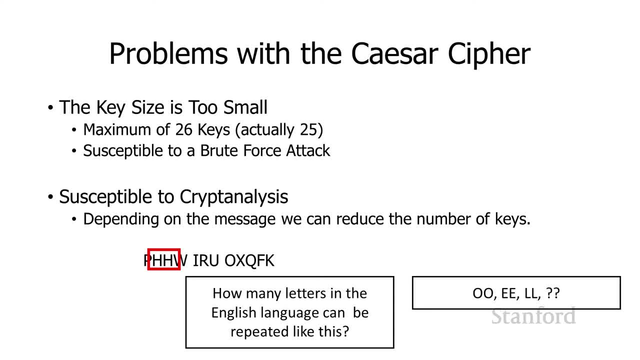 but there aren't that many of them Offhand. there are a lot of letters. There are a lot of letters. You can have two O's next to each other, Like, look, you can obviously have two E's next to each other. 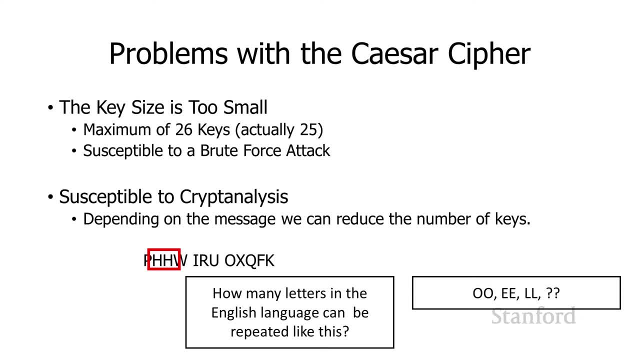 I think you can have two L's next to each other, But there aren't that many letters which you can have two of next to each other and it still be a word in the English language And, moreover, this particular message doesn't have this particular weakness. 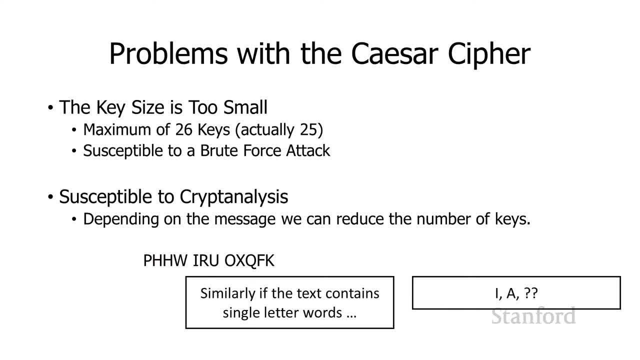 But if we have a message that has a word with a single character in it, there's also a very limited number of messages that can only have a single character in it, like I or A, And so if we're Caesar's opponents and we're intercepting a bunch of these messages, 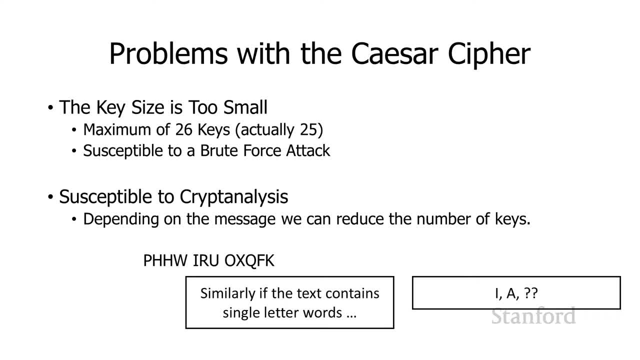 over time, we're going to see messages with these pairs of duplicate letters. We're going to see messages with single letter words And over time, we're going to be able to reduce the amount of possible keys far below the original 26.. 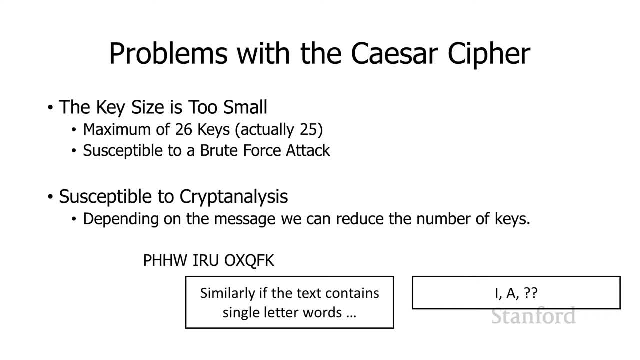 And so the Caesar cipher is just saying: this seems super, super weak And it's a little scary to believe that. And apparently this is true. This was used by Julius Caesar- Shocking. I like using it, though, because it's something. 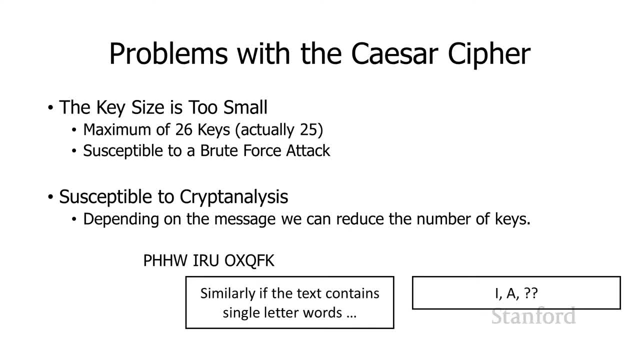 that students can look at and they're like, OK, I kind of get that. And so the same general process is going to be used with real modern ciphers, although the conversion to the ciphertext is going to be much more complex and mathematically based. 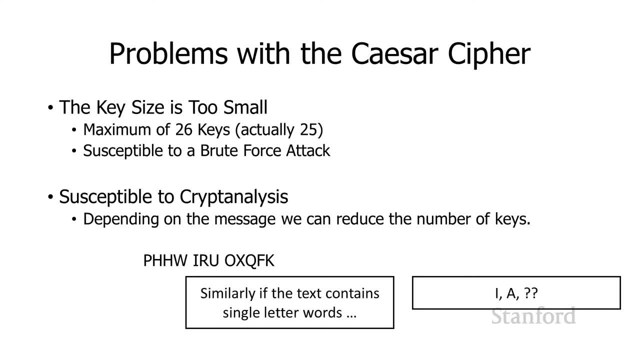 If we look at this, he's just going to say, OK, I'm going to use this, I'm going to use this. If we look at the Caesar cipher, there's actually two different things that are keeping these messages safe. The first one is the number of keys. 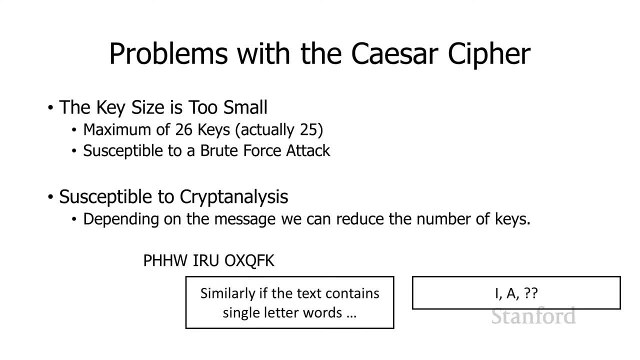 And, as we saw, that's really weak with the Caesar cipher, Although in a modern cipher, that is really the thing that's keeping you safe. You just need a really big key. And the second thing is what the algorithm is And presumably what was keeping the Caesar cipher safe. 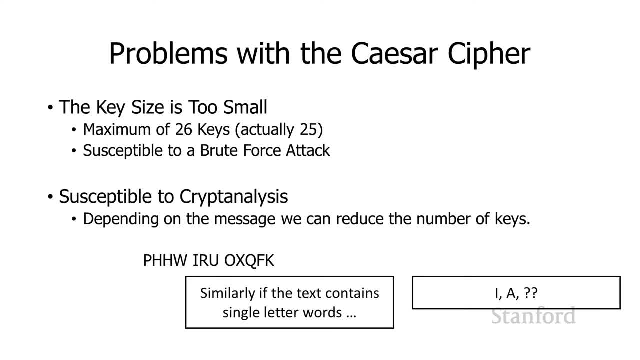 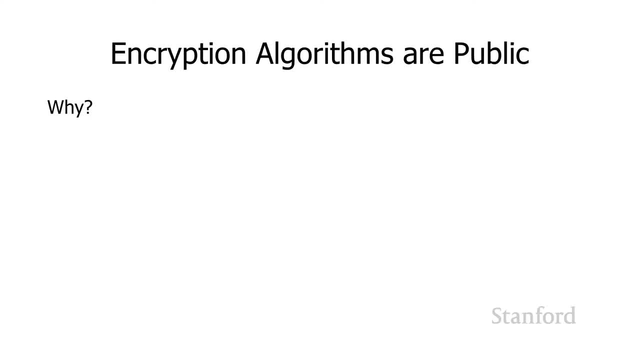 was the algorithm. People didn't realize that this was a shifting algorithm And so they just looked at the message and they just thought it was gibberish And they didn't know how to break the code. But it might surprise you to learn. 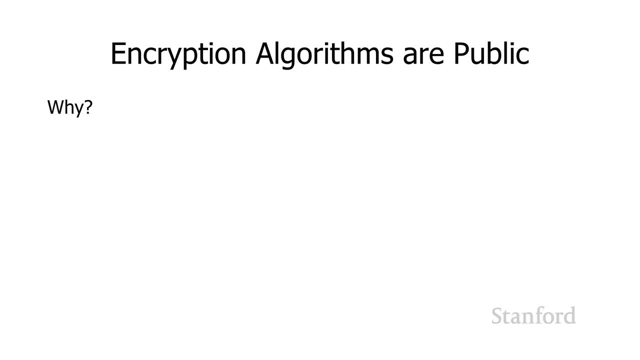 that modern encryption algorithms are all public, So if you want to know the algorithm being used to send encrypted traffic on the internet, well, it's publicly available and you can take a look at it. Why do we tell everybody what algorithm we're using? 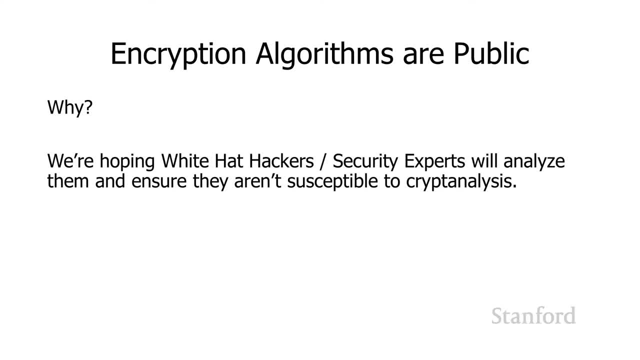 Well, the hope here is that we're concerned that the black hat hackers, the bad guys, are going to be trying to break these algorithms And steal all of our information, And the hope is that the white hat hackers are security experts. The good guys are going to analyze our encryption. 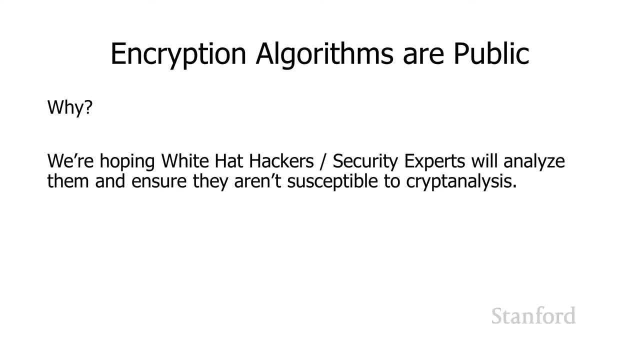 algorithm and determine if they're susceptible to cryptanalysis, And actually Stanford's been involved in several of these efforts, And there are encryption algorithms that were formerly used that are not being used anymore because of work by Stanford computer scientists. So there you go. 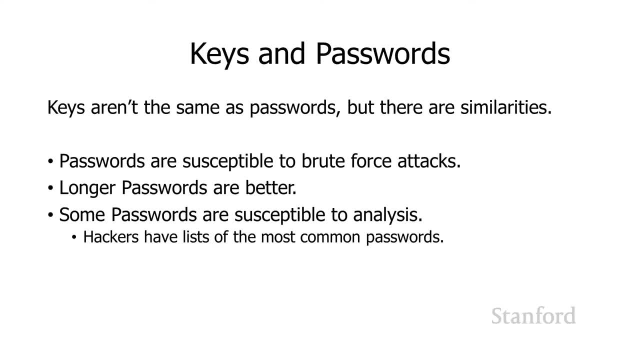 White hat hackers in action. One thing I should mention is that a lot of the things that I say about keys are actually also true of passwords. So keys and passwords aren't the same, but there definitely are strong similarities. So passwords like keys, are susceptible to brute force. 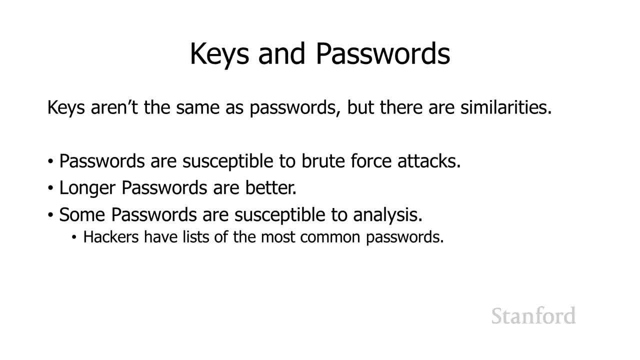 attacks. So with the key, you try all the different combinations With passwords, you just try all the different combinations of letters or letters and numbers until you hit the one that matches the person's original password. And as with the keys, where the problem with the Caesar cipher. 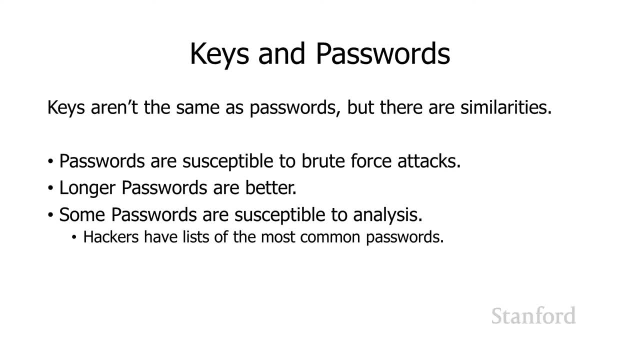 is there are only 25 or 26 keys with passwords. longer passwords are much better, But also passwords are susceptible to analysis And there are certain passwords that are nice and long but that are used by a lot of other people. 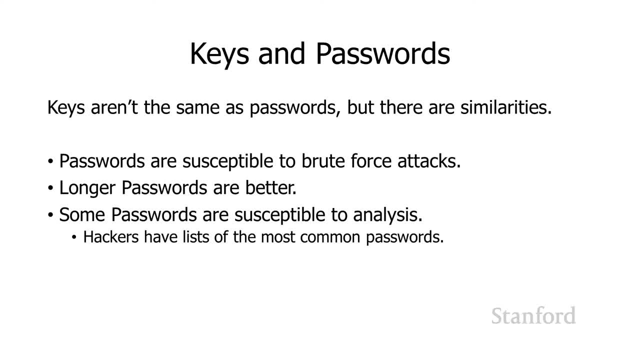 And so that would be a really bad idea to use. those Hackers have a list of the most common passwords, So you really want a long password that it's completely random. We'll talk more about passwords in another lecture, But I just know usually when I'm talking on this subject. 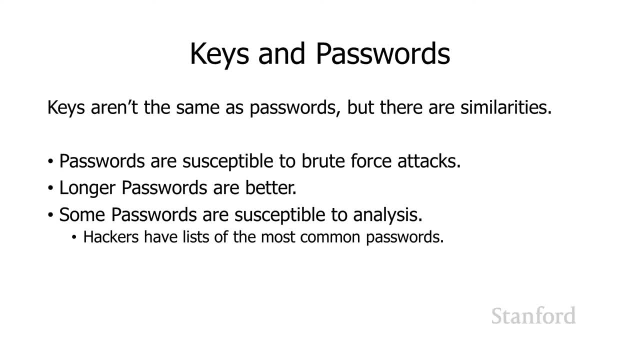 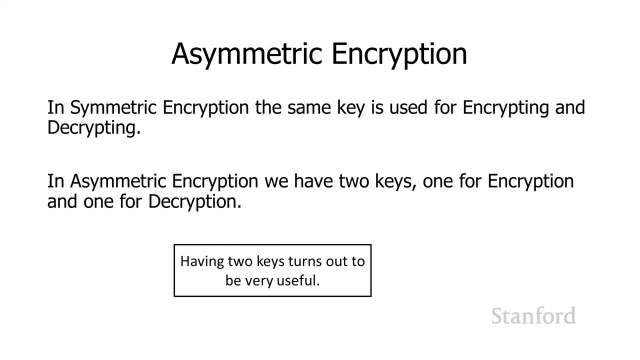 the students get a little confused, because some of the things that we say about these keys seem to be related to passwords, And, yes, there are strong similarities between the two. All right, so the Caesar cipher is what we refer to as a symmetric encryption text. 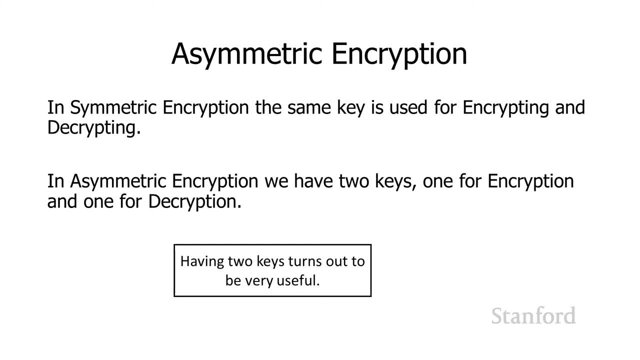 And symmetric encryption. the same key is used for encrypting and decrypting, So with the traditional Caesar cipher, as used by Julius Caesar, the key is 3.. So both the person who's encoding needs to know that they're shifting it by 3.. 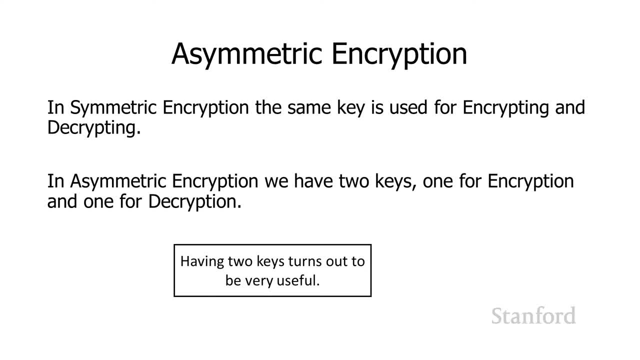 And whoever receives the message knows that they need to decrypt it by shifting back by 3.. So the same key is used for encrypting and decrypting. There's another encryption technique, called asymmetric encryption, where we have two keys. One key is used for encrypting and the other key 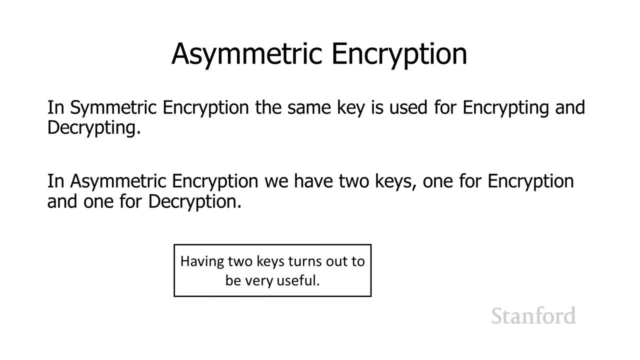 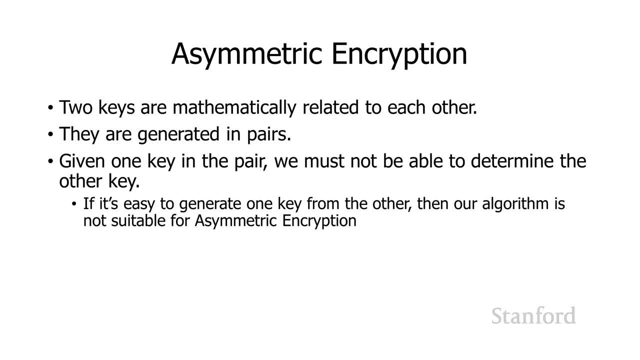 is used for decrypting And it turns out having two different keys is super, super useful. Now the two keys have to be mathematically related to each other and they are going to be generated as pairs, And if we have one of the keys in the pair, 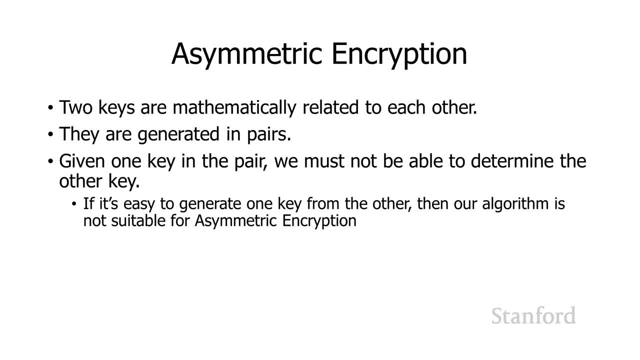 we can't be able to determine the other key in the pair easily, Because if I can get from one key to the other key, these keys are going to be useless for asymmetric encryption. So they're generated together at the same time, But if somebody gets a hold of one of the keys, 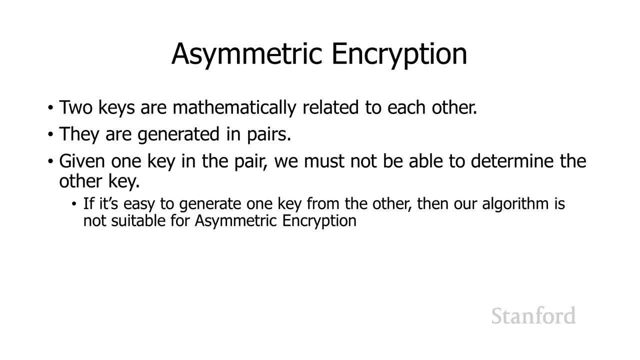 but doesn't have the other key, they can't be able to reverse engineer it to figure out what the matching key is. That would be bad, And if they are able to do it, then we're completely vulnerable. So symmetric encryption has been around for pretty much. 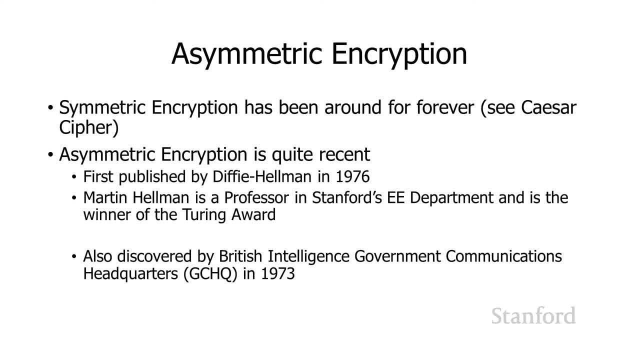 forever, as we've seen from our example of the Caesar cipher, Asymmetric encryption, on the other hand, is quite recent. It was first published by Diffie-Hellman in 1976. And the Hellman in Diffie-Hellman is actually. 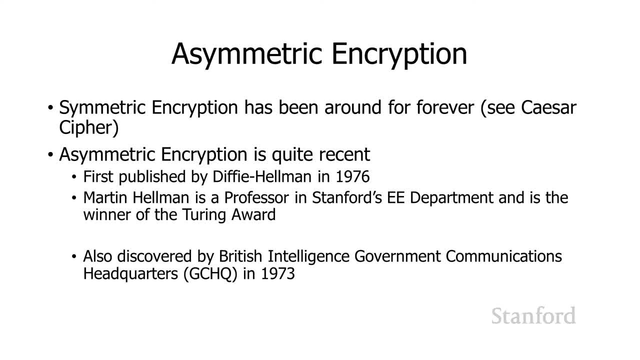 Martin Hellman, who's a professor in Stanford's EE department and is the winner of the Turing Award, which, you'll recall, is the equivalent of a Nobel Prize in computer science. I guess when Alfred Nobel was creating the Nobel Prize is there was no computer science at the time. 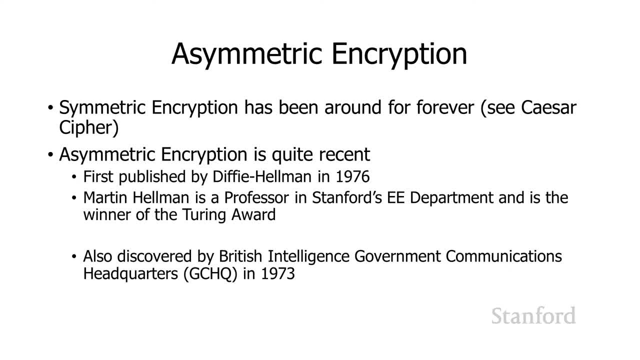 so we didn't get one of them, So we made up our own, which is the Turing Award. And Professor Hellman is the winner of the Turing Award, Turns out. it was also discovered by the British intelligence government communications headquarters in 1973,. 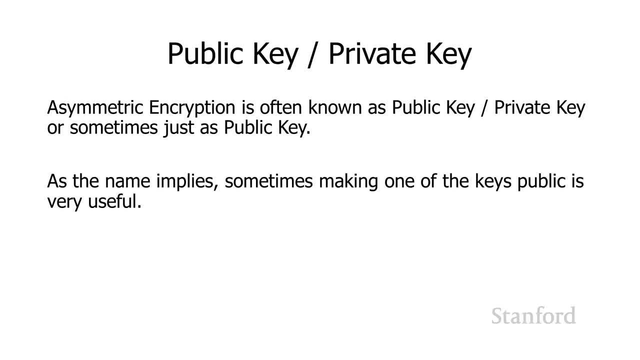 but they didn't publish the work. Asymmetric encryption is sometimes referred to as public key, private key encryption or sometimes just simply as public key, And, as these names apply, making one of the keys public is often very useful And it will allow us to solve a bunch of the problems. 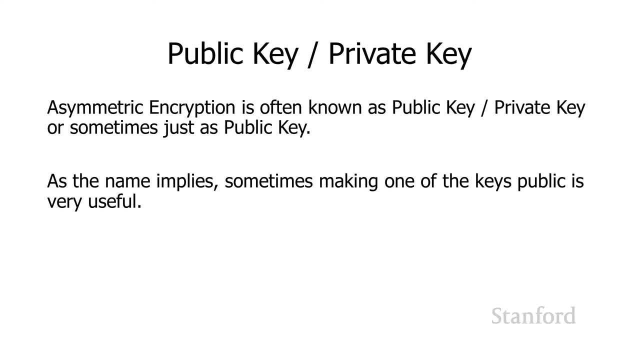 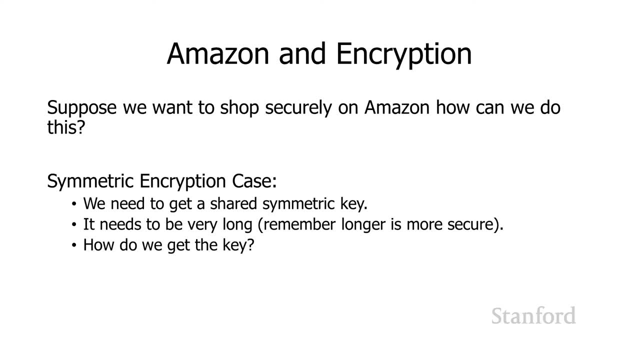 that we looked at when we were talking about network security issues. So one of the problems of symmetric encryption is the problem of how somebody gets a key. So suppose I am communicating with Amazon and I want to communicate with them in a secure manner. I'm going to provide them with information like my credit card. 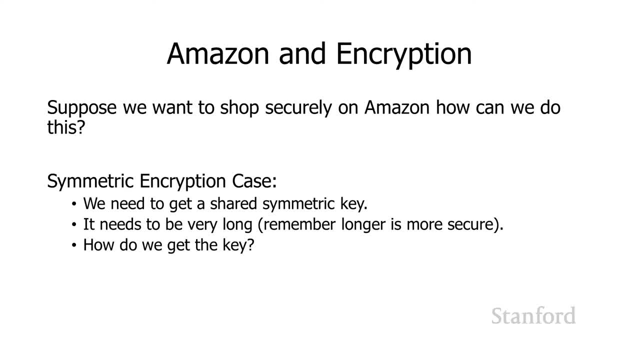 How can we make sure we're shopping securely on Amazon If we've got symmetric encryption? we know we need to have a shared key. We're both using the same key for encrypting and decrypting. We both have that key And it needs to be very long because remember. 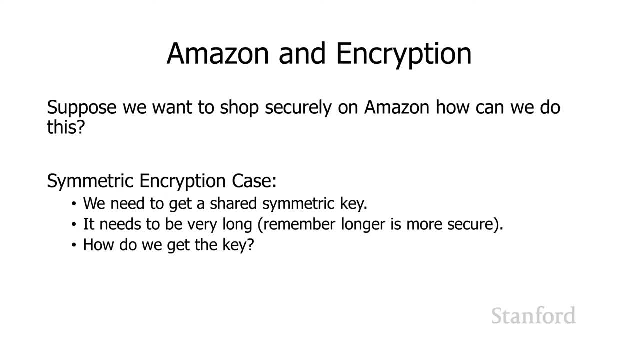 longer is better, Longer is more secure, And so the big question that comes up is: how do I get the key? Well, think about that for a minute. How am I going to get the key from Amazon? Well, one obvious thing is they could email to me. 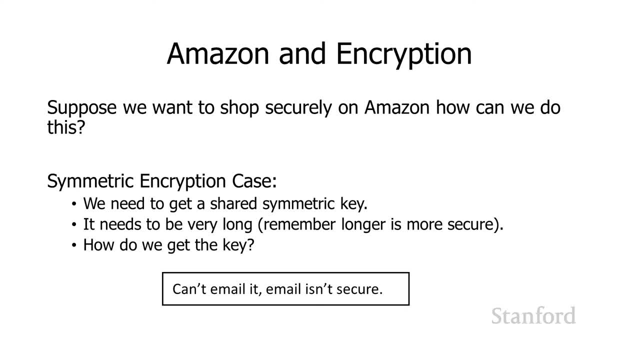 That turns out to work, Because email is not secure And in fact I can't think of a good way for Amazon to get that key to me other than through snail mail. But snail mail is sending to the US Postal Service. 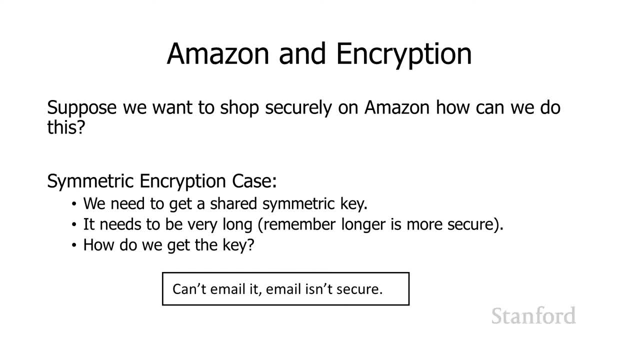 That's a really bad idea from their standpoint. I mean it will work, But that means I would put a bunch of stuff in my shopping cart the first time I went to Amazon And I'd be like, OK, I'm ready to check out. 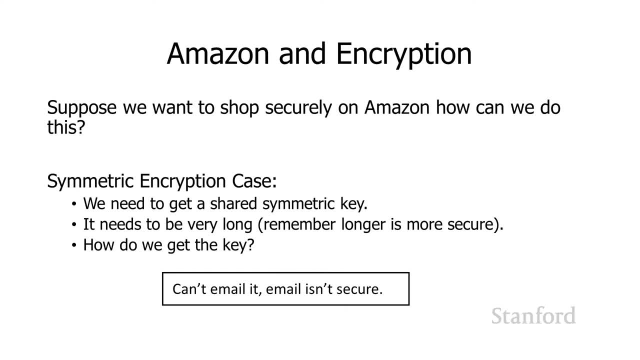 And they'd be like: oh well, we're going to mail you this key through the US Postal Service And it will probably take three days- But it might take longer- And when you get it, you can enter the key into the web browser. 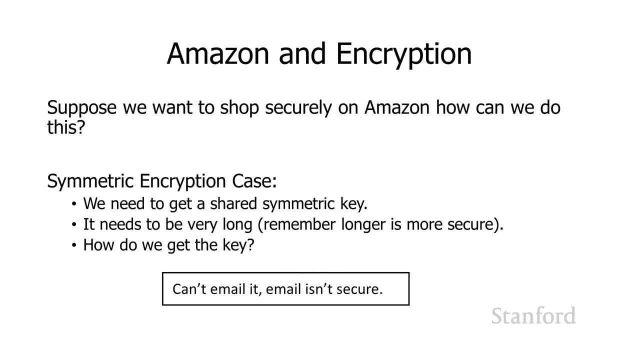 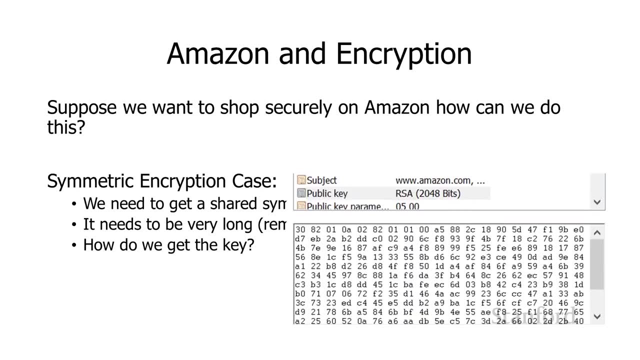 And then you can send us a credit card Like: yeah, I'm pretty sure they would lose a lot of people just at the shopping cart right at that point. The other problem is: take a look at what the key looks like. So this is the actual key that Amazon has. 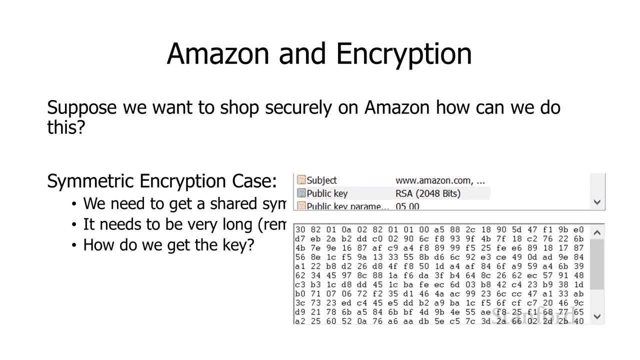 You can see it doesn't actually fit. You can see a little scroll bar there on the right. If Amazon were to make it Mail this to me, it would be on the printed page And I would have to enter in all of these hexadecimal digits. 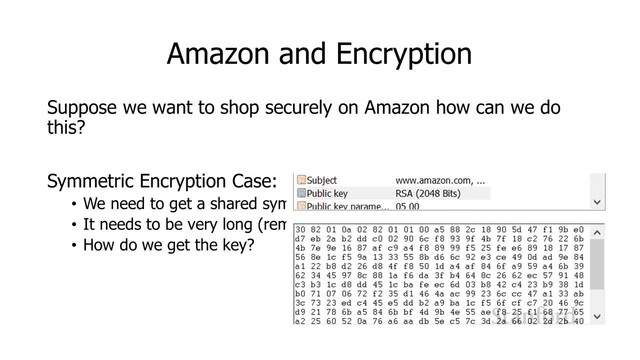 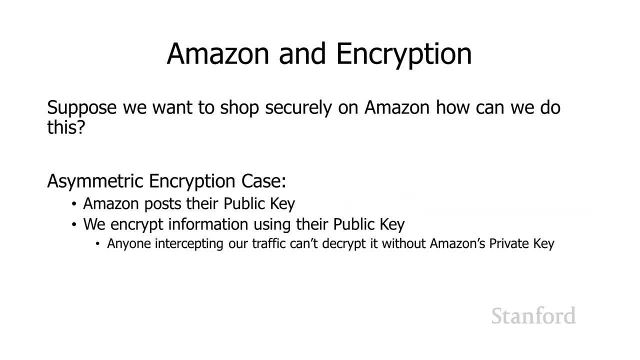 and not get any of them wrong- in order to communicate securely with Amazon using symmetric encryption. OK, this is totally not happening. All right, so how does asymmetric encryption solve our problem? Very easily, Amazon takes one of their keys, says this key is going to be the public key. 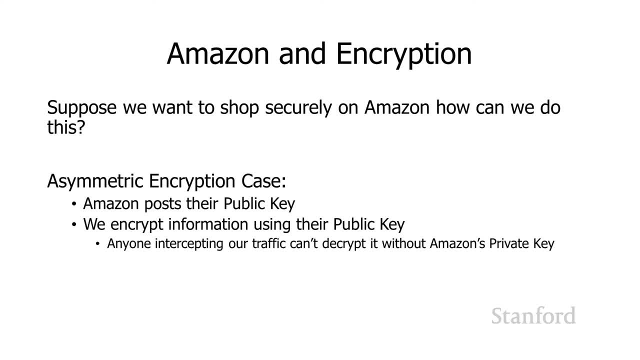 and they just put it up on their website. In fact, we just saw it a minute ago. That's their public key And then when I want to talk to Amazon, I take their public key and I encrypt whatever I want to send to Amazon with that public key. 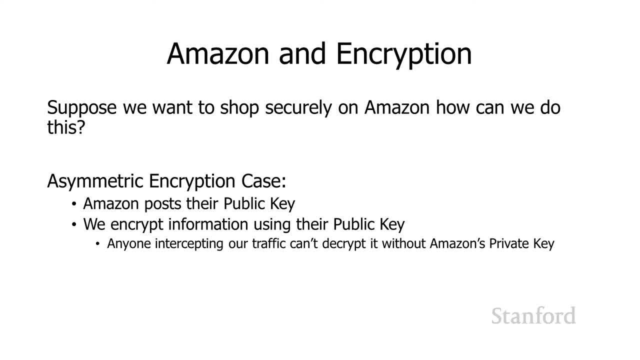 And anyone intercepting our traffic can see that I'm sending information to Amazon. They know it was encrypted with the public key. They also have access to that public key, But that public key doesn't- It doesn't decrypt messages that were encrypted with it. 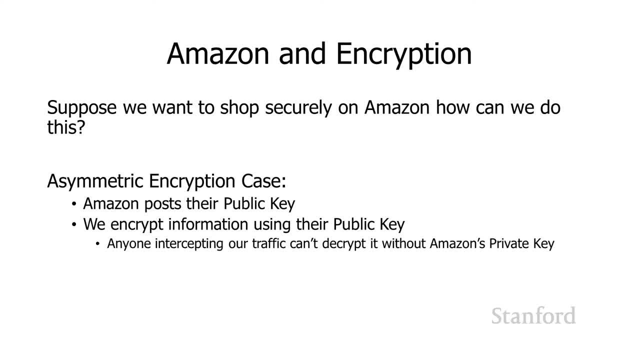 We need the private key in order to decrypt the message. We don't have the private key, And as long as Amazon keeps their private key private, I can encrypt messages and send it to Amazon and nobody else can read it. So we are now able to communicate with Amazon. 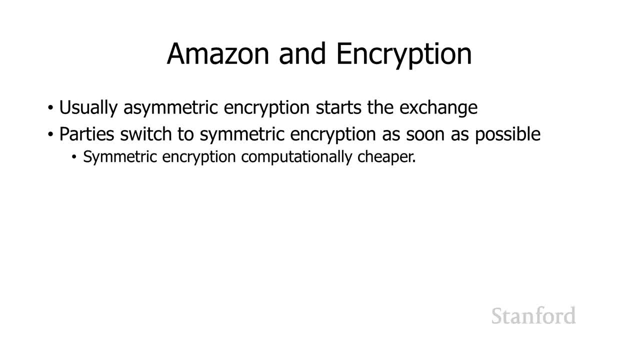 in a secure manner. Now, usually what's going to happen with websites like Amazon? all the other websites work the same way. I'm going to start off with an asymmetric encryption, because they're going to provide me with their public key And I'm going to encrypt something and send it to them. 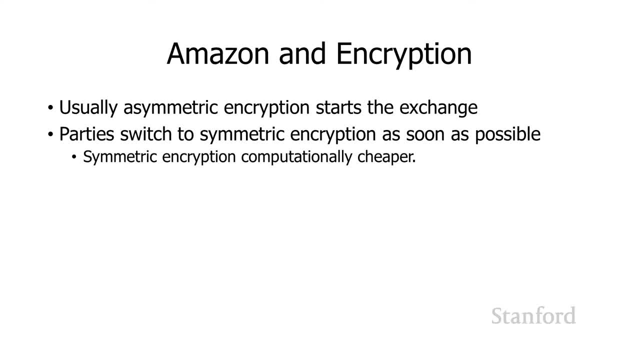 And they're the only ones that are going to read it, because they're the ones with the private key. But as soon as we can, we're going to generate a symmetric key that only the two of us use, only the two of us know. 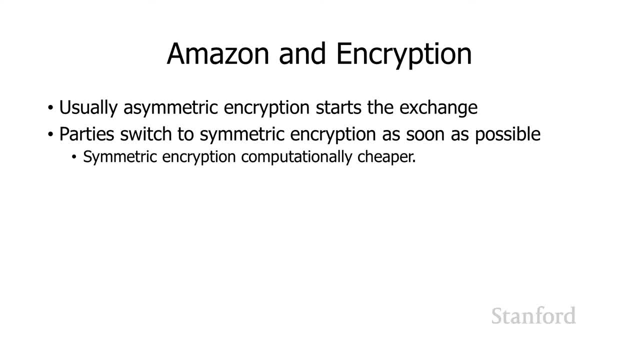 And that's what we're actually going to use for regular communication. because, it turns out, symmetric encryption is computationally cheaper than asymmetric encryption. Since their web server is decrypting all these messages, anything they can do to reduce the load on the server is going to be better for them. 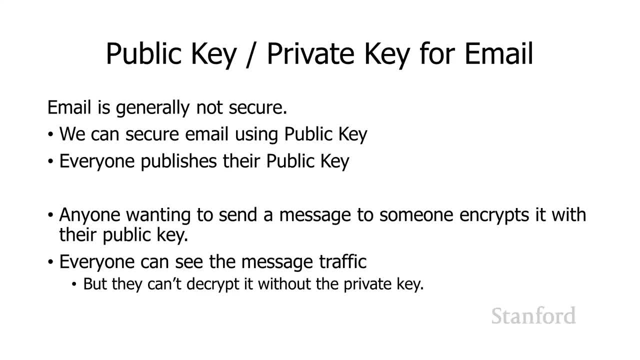 It's going to be cheaper for them. OK, I mentioned that email is not secure, generally not secure. It is certainly possible to create a secure email system using public key, private key, And in fact, there is a system out there. 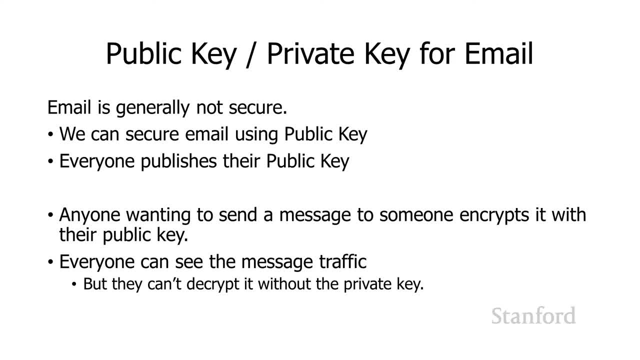 It's just not very widely used. OK, so how do we create a secure email system using public key? Well, basically, everybody just publishes their public key And then if somebody wants to send them a message, they just take that public key. 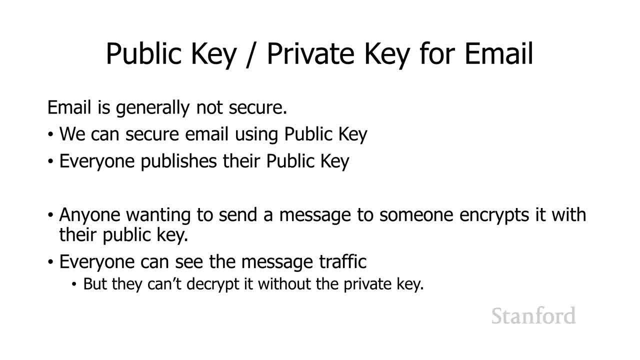 They encrypt the message with that public key. They send it through the internet. Everybody can see all the traffic sent through the internet, But if somebody sees that message on the internet, it's encrypted with a public key. They also have access to the public key. 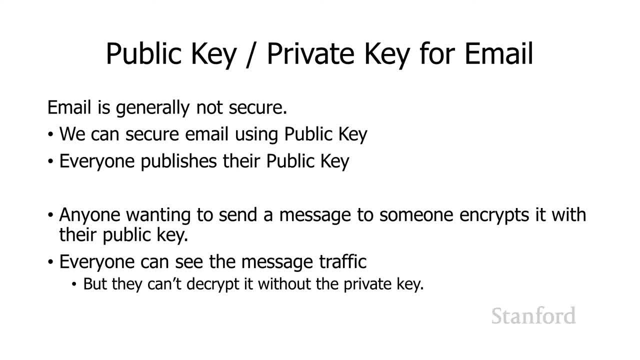 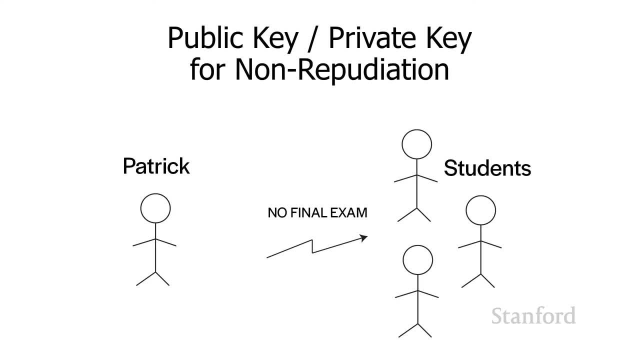 but they don't have access to the key that they need to decrypt it. That's the private key, And so the email is secure. Public key- private key can also be used for non-repudiation. So here's your call. 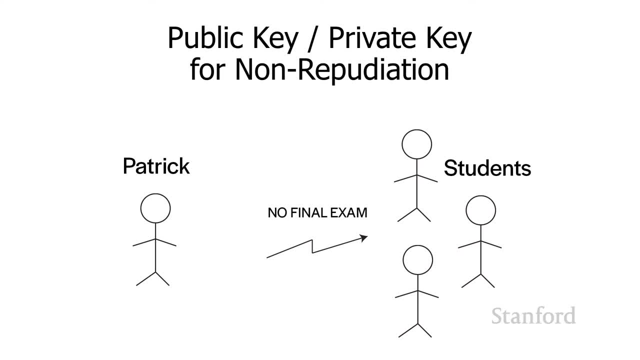 This is our non-repudiation example from last video. So suppose I send out a message I say no final exam. Maybe I'm drunk or something And on a lark I decide to send out this: no final exam message. 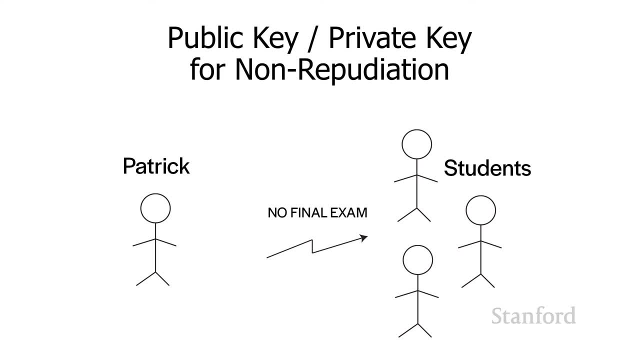 And then later the next day I'm like: oh God, did I actually send out a message? There was no final exam. Oh crap, I didn't mean to do that. I'm going to take it back. I'm going to tell them that wasn't me. 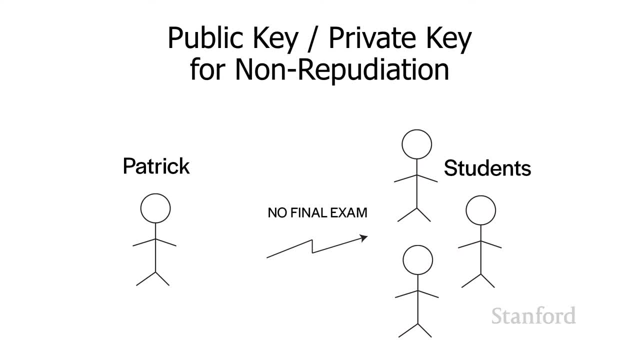 Somebody else must have been Maddie. That actually is not a very good example, because if Maddie actually has access to my computer, she could totally send it in a way that would violate our little example here. So anyway, so I'll talk about that in a minute. 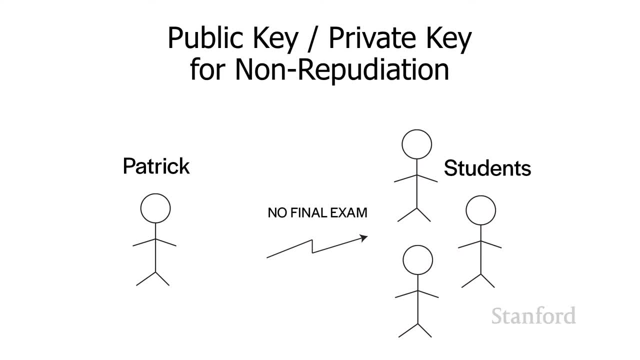 when I tell you how this all works. All right, so the way we have non-repudiation is, if my system is set up So that when I send that message- no final exam- I actually encrypt no final exam with my private key. 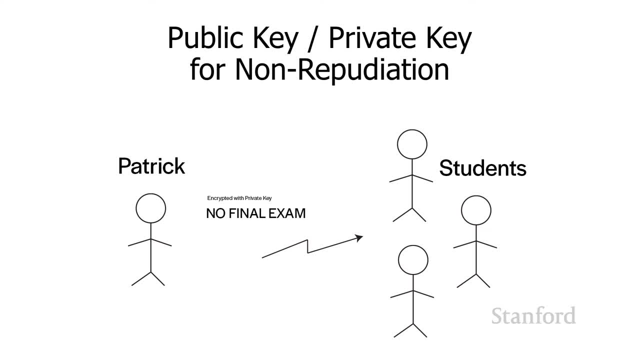 And you guys all receive it and you decrypt it with my public key. Now you can be like Patrick. you must have sent that message, because only you have the private key that could be used to encrypt the message in such a way that we can decrypt it with your public key. 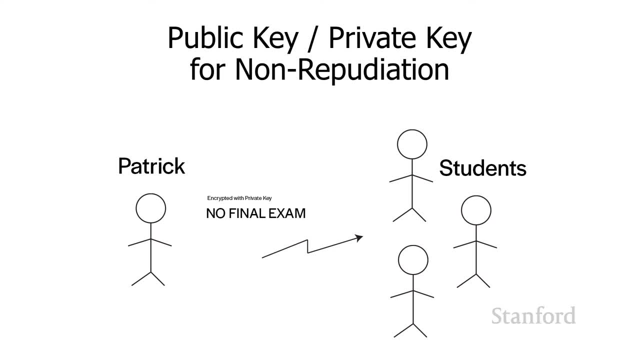 So therefore, you can't repudiate it. You must have sent this OK. going back to our example, Maddie. if Maddie actually has access to my computer, she's sleeping under the coffee table right now. If Maddie actually has access to my computer. 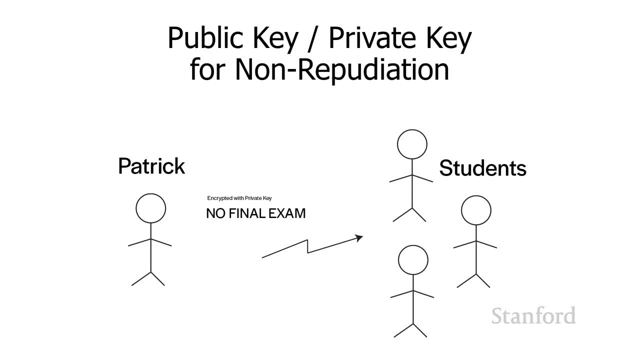 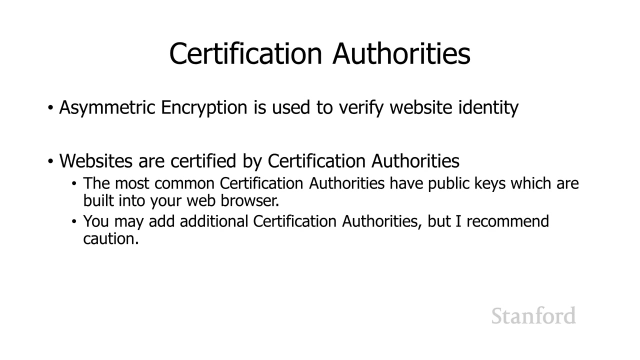 and my private key sitting there on my computer and probably my whole email system set up to use the private key, she could totally send the message. So basically, this whole system is only as secure as your private key is secure. OK, Asymmetric encryption is also used to identify websites. 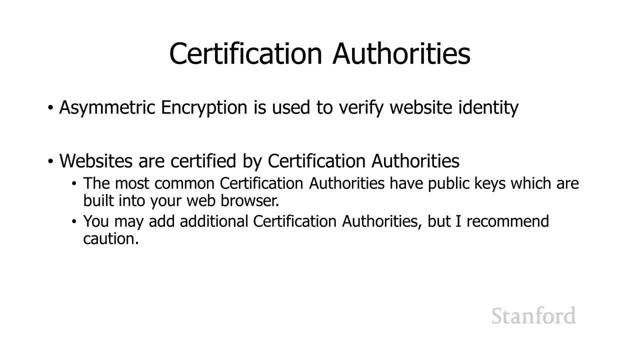 The way this works is that there are a number of what are referred to as certification authorities that are responsible for certifying websites. The most common certification authorities have public keys which are built into your web browser. It's also possible to add additional certification authorities by explicitly adding their public keys. 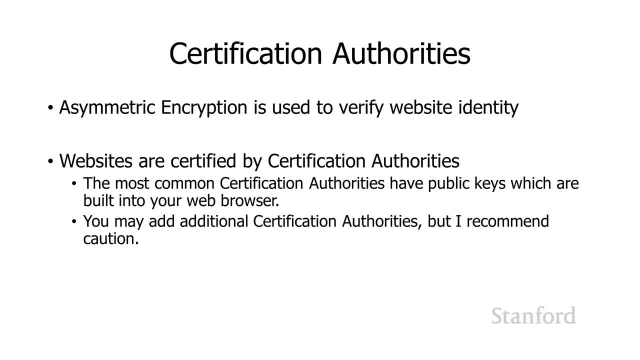 to the web browser. I don't recommend doing this In general. So if you go visit certain websites, you may get a message that, oh, this website is certified by such and such a certification authority which the web browser doesn't know about. 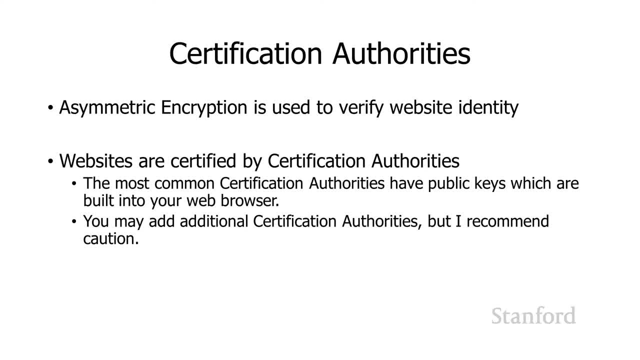 Should I add this certification authority to your list of certification authorities? And, in general, I don't think there are good reasons for a website to not use one of the standard certification authorities at this point. So just be aware, if you say yes, that 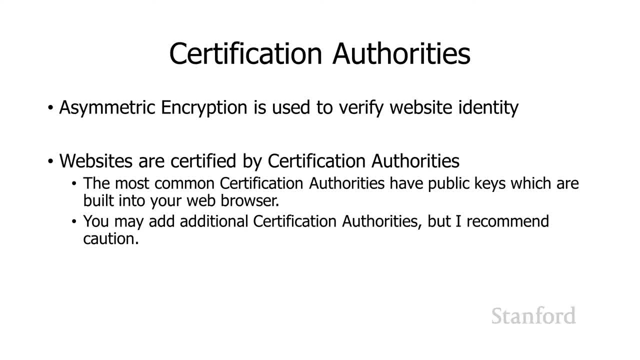 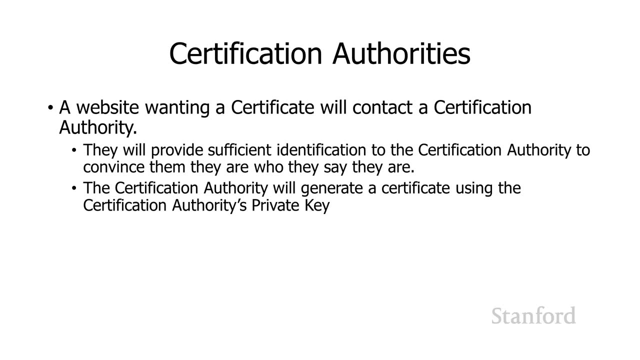 means other websites certified by this potentially sketchy certification authority are also going to be assumed to be legitimate by your web browser, And that may not be something that you want to do, So be cautious adding additional certification authorities to your web browser. So the way this is going to work is a website that 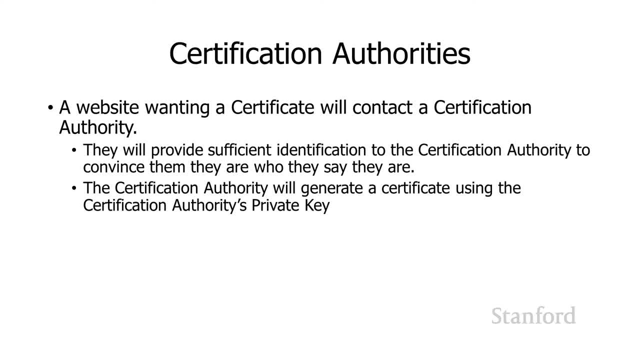 wants a certificate is going to contact the certification authority And they will provide sufficient identification to the certification authority to convince the certification authority that they are who they say they are, And then the certification authority is going to take their information and generate a certificate using the certification authority's. 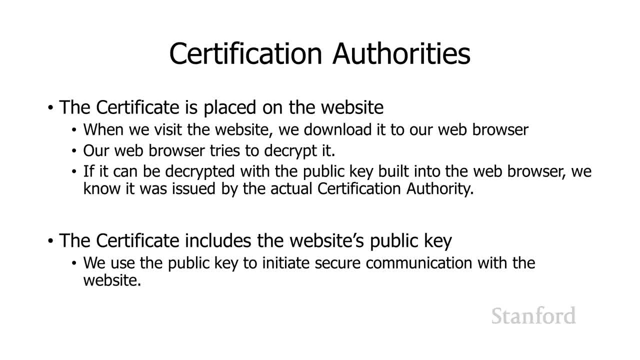 private key, And so you have the public key built into the web browser And the certification authority has the private key used to generate the certificate. The certificate is going to be placed on the website, And when we visit the website we will download the certificate to the web browser. 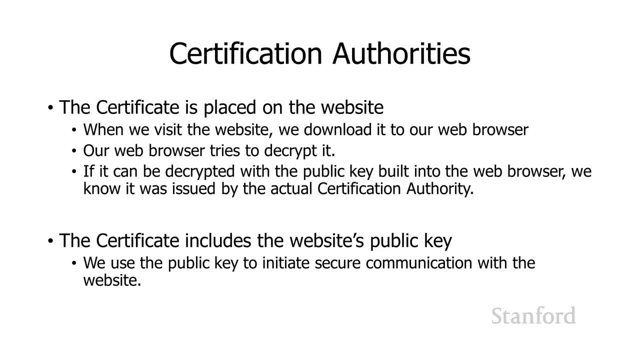 The web browser will attempt to decrypt it, And if it can be decrypted With the public key built into the web browser, then we know it was actually issued by the certification authority. The certificate includes the website's public key, And we use the public key to initiate communication. 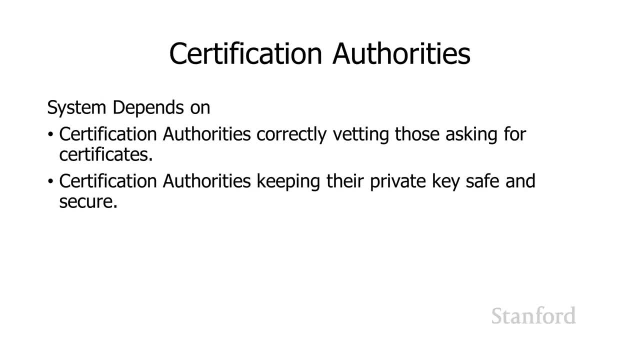 with the website, Notice that this system does depend upon the certification authorities correctly vetting those who ask for certificates and also keeping their private key safe and secure, And it turns out that, sadly, both of these have failed at various points With this certification authorities. 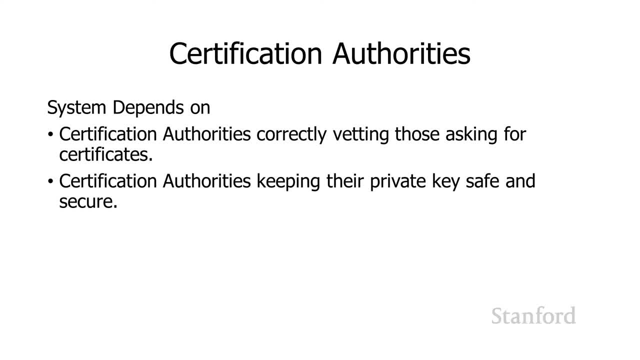 there's been at least one case that I'm aware of where a certificate was authorized and given to somebody claiming to be Microsoft And it turned out they weren't Microsoft, And there's also been a case where the certification authority itself was hacked and their private key was stolen. 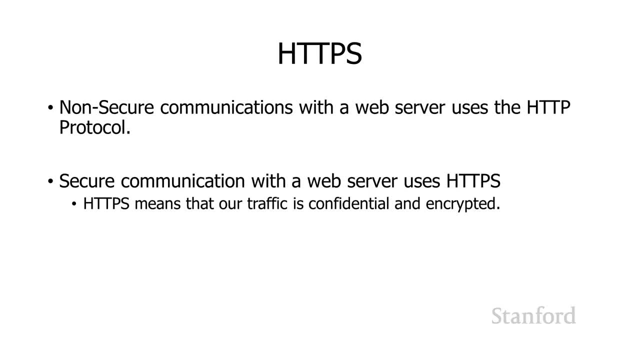 So great job, guys. When you are communicating with a website that has a certificate and is You're going to be communicating using HTTPS instead of HTTP? So standard non-secure communications on the web uses HTTP. Secure communications uses HTTPS, which is a secure variant of HTTP. 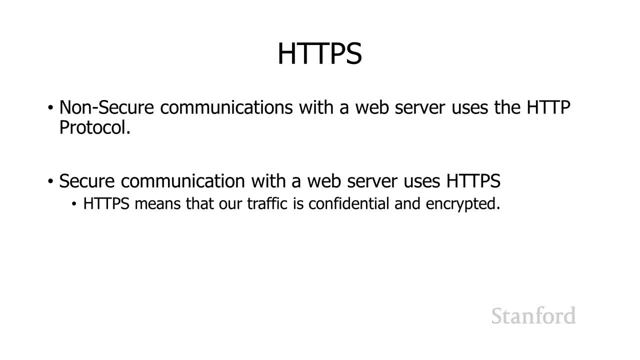 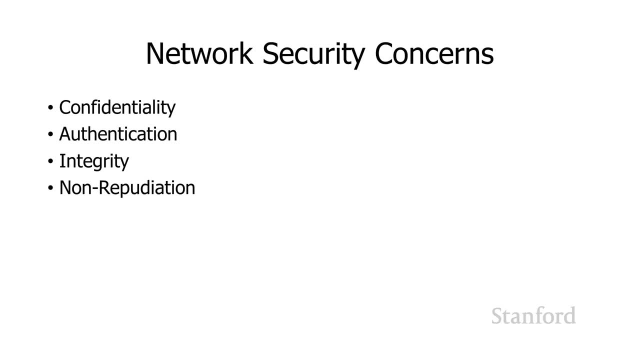 And when we are using HTTPS, that means that all of our traffic to and from that website is being encrypted. OK, let's go back to our list of notes. Network concerns that we had before. So confidentiality: being able to communicate in a secure manner. 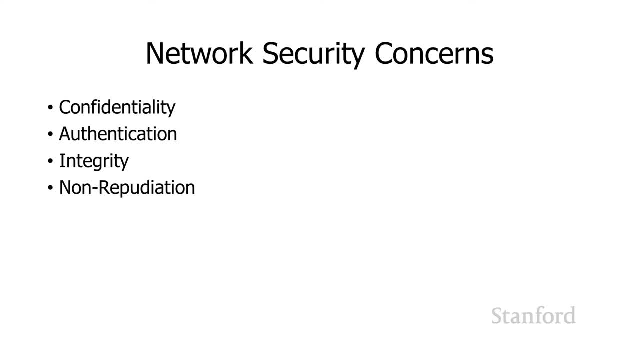 such that if somebody is trying to eavesdrop, they can't read our communication. Well, we've seen that both symmetric and asymmetric encryption takes care of that Authentication. we've just seen that with the certification authorities. The certification authorities use public key, private key. 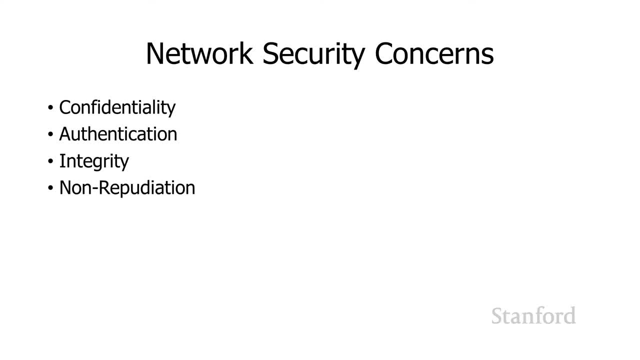 in order to provide certificates that guarantee that a website is who they say they are. Non-repudiation: we saw that public key, private key- could be used to set up a system where people could not repudiate actions that they had taken. 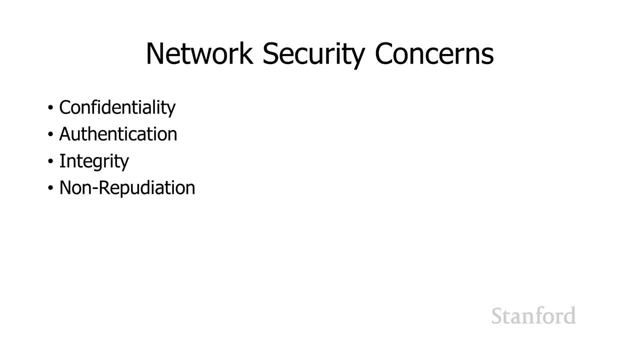 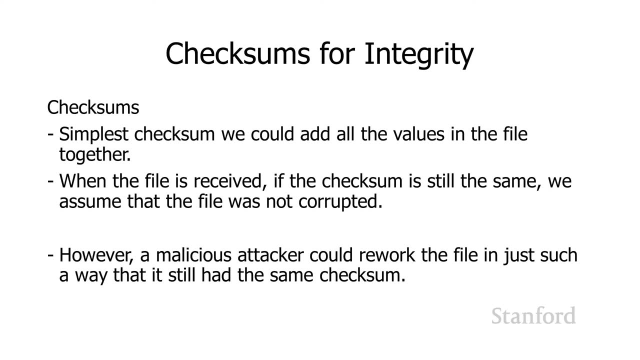 And then that leaves integrity, which we haven't talked about yet. So let's take a quick look at integrity. The simplest way to generate integrity is to use a checksum And checksum. there's a variety of different ways to do checksum, but the simplest way to do it. 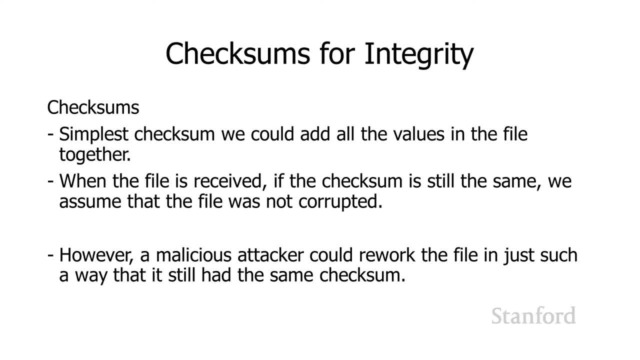 is to use a check sum, And the easiest way to do it- that I think students understand intuitively- is you just take all the different values that are contained in the file, treat all those bits as numbers and add all the bits together. Now it's going to come up with a really big number. 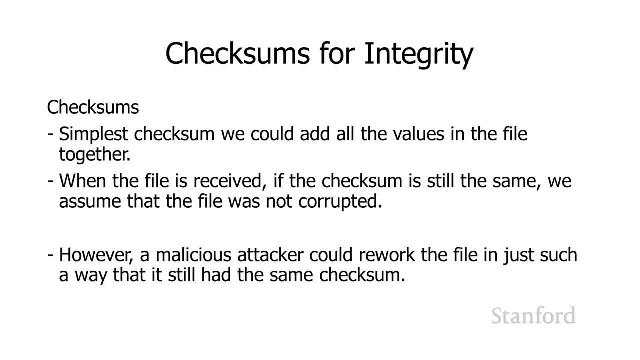 so you probably want to chop off a whole bunch of the high end bits And basically do a modulus. If you're familiar with the modulus, it's sort of a remainder, integer remainder, And then you go ahead, You add a value and use it as your checksum. 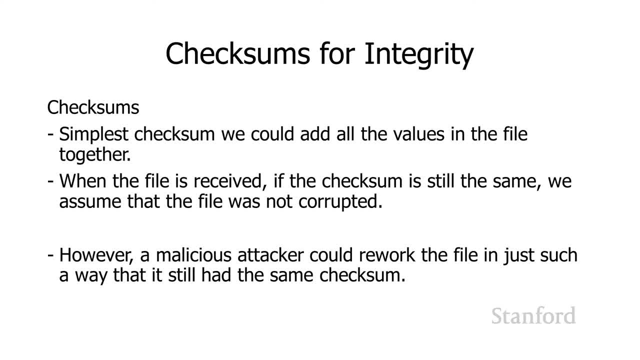 All right. so the way this is going to work is if you transfer, say, a file over the internet, originally, the person that created the file is going to create that checksum. They're going to either include it with the file or they will send it separately from the file. 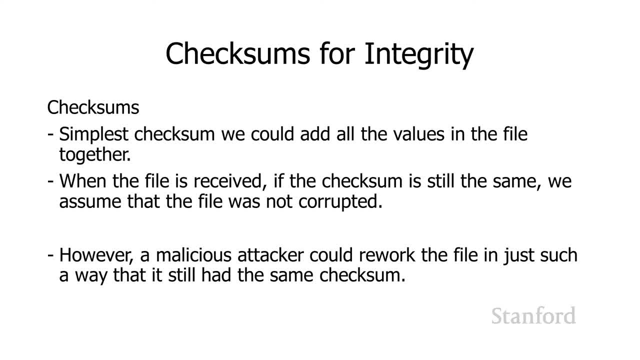 Your computer will receive the file. It will go back through and add everything up to see what checksum it gets, And if the two checksums match, then you know that there's a good chance that the file was not in fact corrupted. 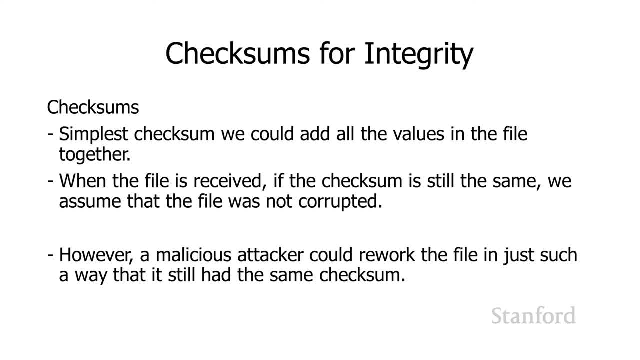 Now it's possible for the file to get corrupted in just such a way that the checksum is still the same, So that is a possibility, but it's unlikely. The problem with checksums, though, is since it's pretty easy to understand how the checksum was. 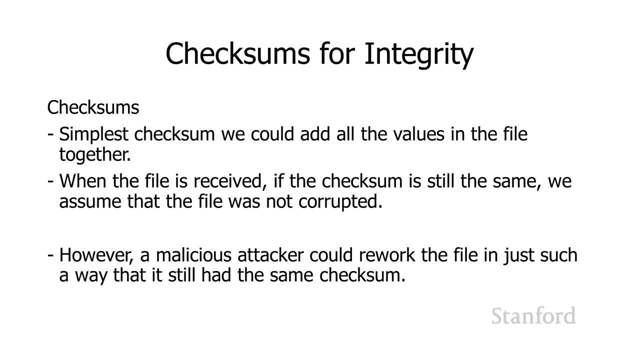 generated. it's also pretty easy to reverse engineer Things so that you manipulate the file in just such a way that the checksum remains the same, So this is actually kind of a problem. I should also mention that you may run it to checksum if you download a zip file. 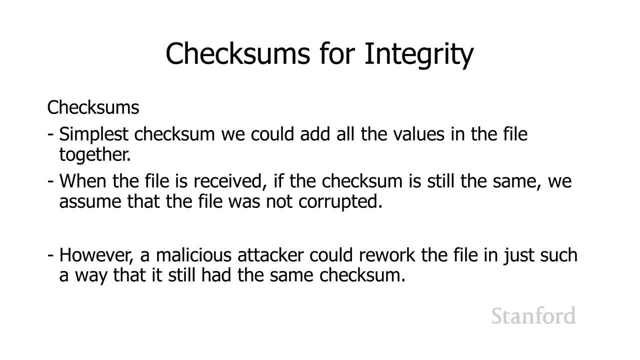 You will occasionally run it to zip files where it says there's a checksum error. and so that's what's going on with those. It's saying, hey, we calculated the checksum when we generated the zip file, And now, when we're unzipping it, 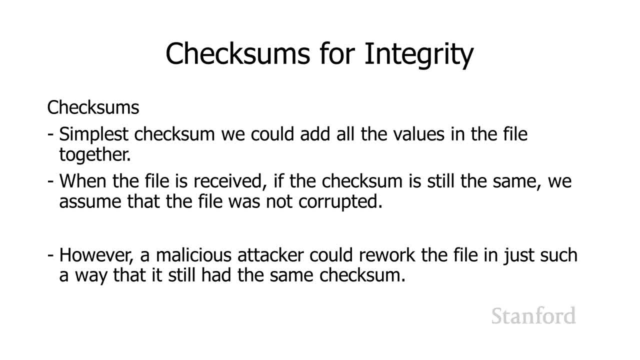 we're double checking the checksum and they don't match. So something went wrong here. Either it was you downloaded over the internet and some of the bits got twiddled, or maybe somehow got corrupted on one end or the other end, But somehow we know that the checksum is not. 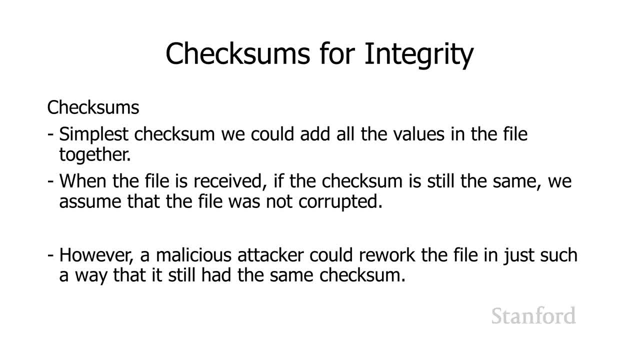 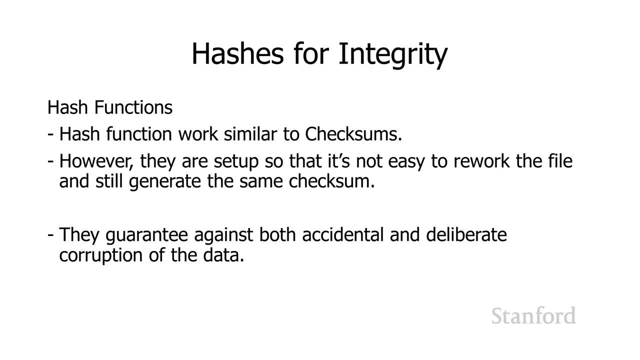 the original checksum for the files when we originally generated the zip file. so something is wrong here. So that's probably the most likely place you're going to run it to checksum, All right. so, as I mentioned, I'm a malicious attacker, can manipulate the file in just. 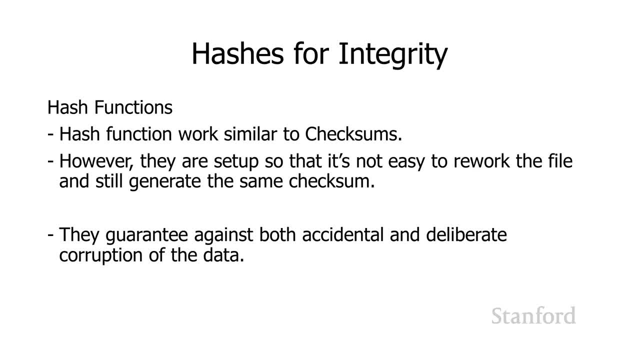 such a way to maintain the checksum. So there's another technique we can use, called a hash or a cryptographic hash. These work similar to the checksum, but they work in such a way that it's much more difficult for somebody to try and manipulate the file in such a way that we end up. 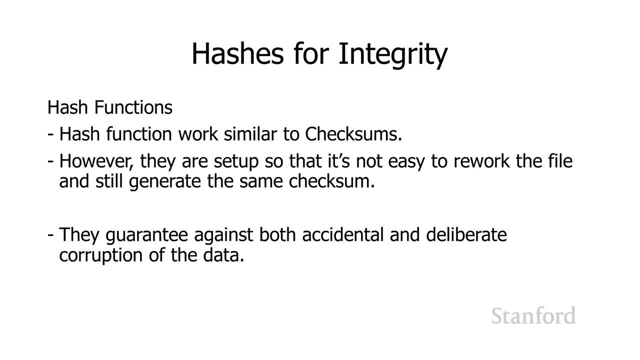 with the exact same hash. So these are going to guarantee from both accidental changes, which is what our checksum did, but they will also guarantee against deliberate corruption of the data. You will occasionally run into these when you download things from websites, particularly software that's open source. 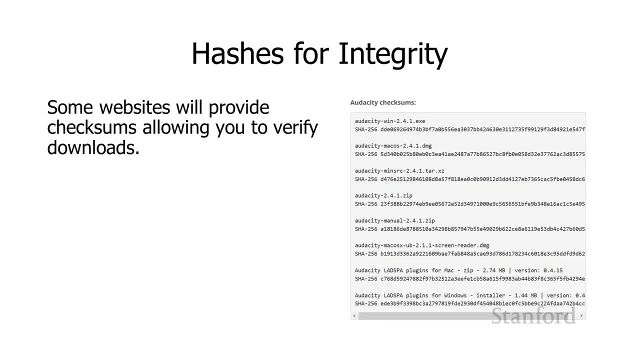 So here I used a program called Audacity much early in the quarter- actually the first week of the quarter- when we were talking about computer music. It was a program where I was playing music to the computer and it was showing us what the waveform looked like. 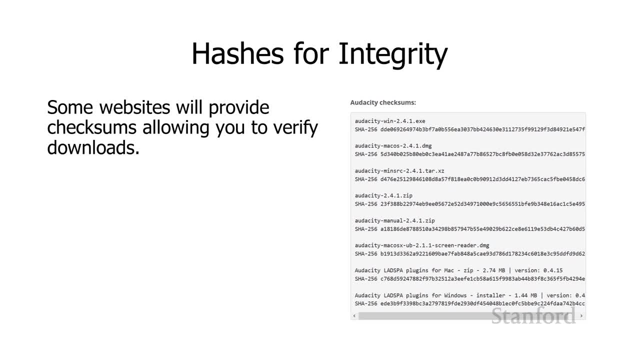 If you go to the Audacity website, they don't actually host the Audacity files themselves because it costs a lot of money to serve up copies of the Audacity files to everybody that asks for them. So instead they have a bunch of other people. 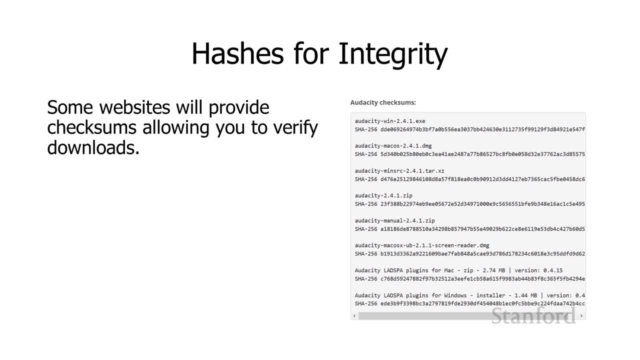 you can download the files from, And they want to make sure that whoever gives you a copy of the Audacity source files has not somehow corrupted it and added in some sort of malicious thing in their code. We'll talk about the different malicious things you could put in the code actually. next lecture. 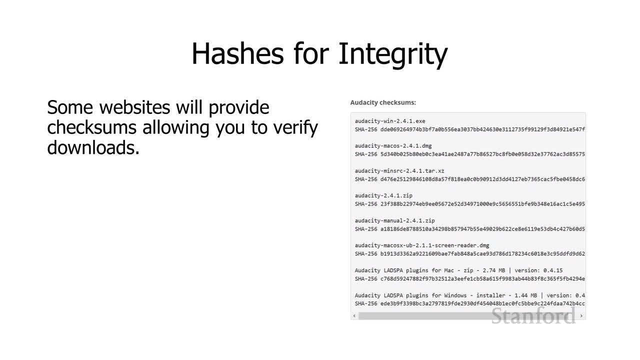 OK, OK, OK. So what they've done is they've provided the different checksums, And so you can see they have a whole bunch of checksums, because there's a copy of Audacity for Windows, there's a copy for Mac, there's a copy for Unix. 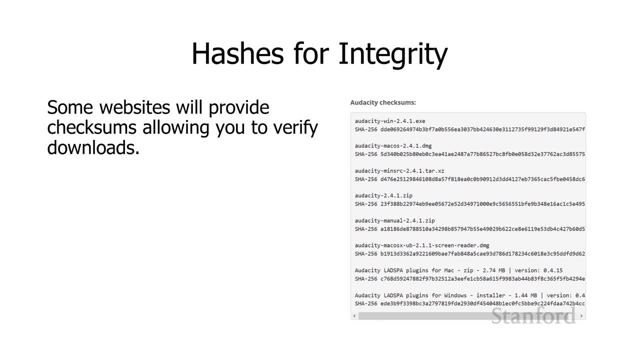 and so on and so forth, And so each of these is a different file, It has different code involved and therefore it has its own checksum, And so the idea here is that you would download the file from a third party. You would get a hold of that file. 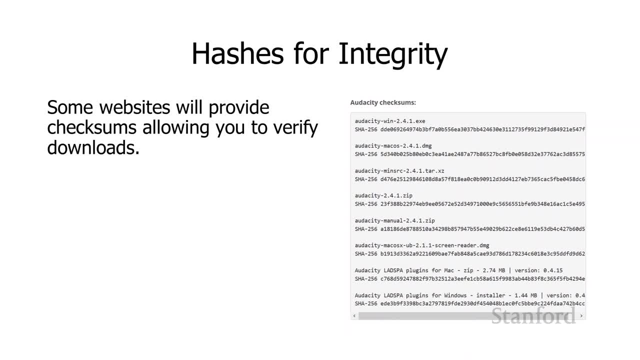 and you would run something to generate the cryptographic hash. So it turns out it is marked as checksums, but these are actually using a cryptographic hash technique, That sah256 that you see in front of each of these checksums. that is actually the specific cryptographic hash function. 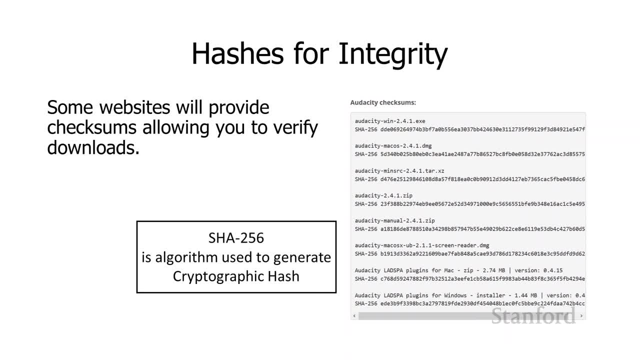 that you need to run in order to get that number back. So you would go ahead and download one of these files from either from Audacity And Audacity itself, which I think redirects to other people's websites, or maybe you get it from a friend or somebody. 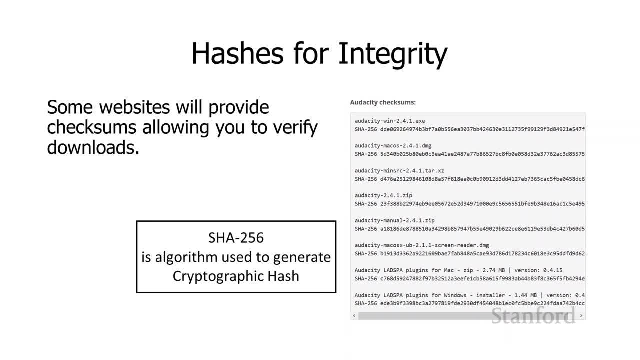 you want to just double check and make sure that this file is in fact what it says it is, And so what you would do is you would take that file, You would run the SHA256 algorithm on it That would generate this big, long number. 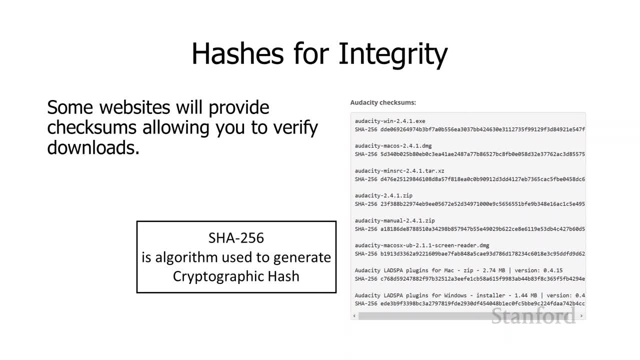 And you would compare the big, long number that the SHA256 generated from the file that you have with the number published on the Audacity website as the correct checksum, And if the two match, then you would have the code. Yeah, That's right. 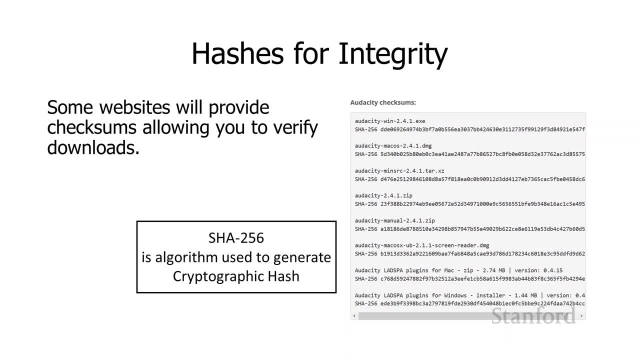 Yeah, match. that tells us that this is in fact the original file that Audacity came up with, And if it doesn't match, that's pretty bad. It could just mean that the file was just corrupted in network transit, or it.